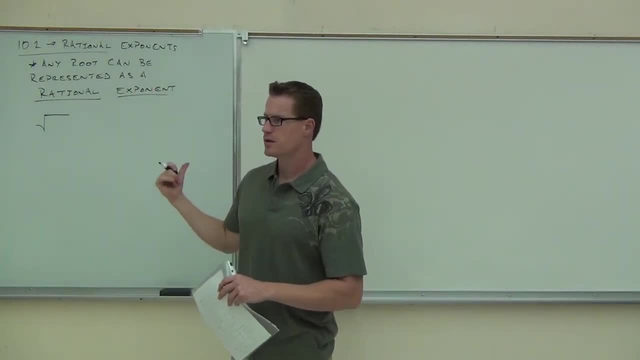 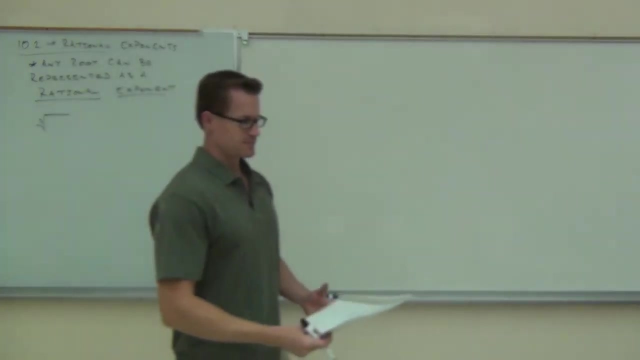 Square root, Square root. And if I had a cube root, what number would I put and where would I put it? Three Right, a little like indices. part a little crotch of this thing. Right, Right, Right there, That little thing. 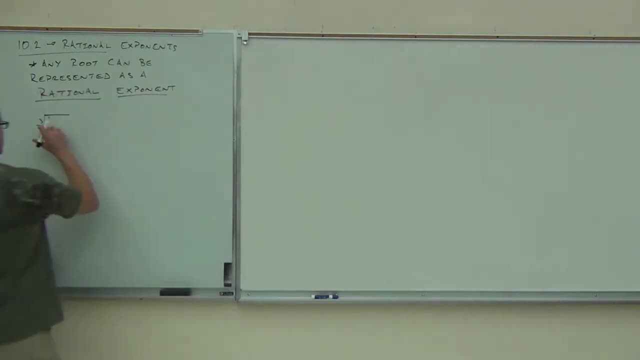 That's where I'd put a cube root. If I had a fourth root, I'd put a number four there, Or an nth root. for any root, I'd put a little n there And whatever's on the inside, we're going to represent that with an a. 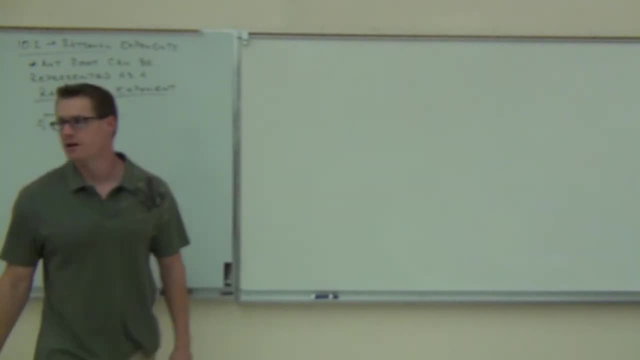 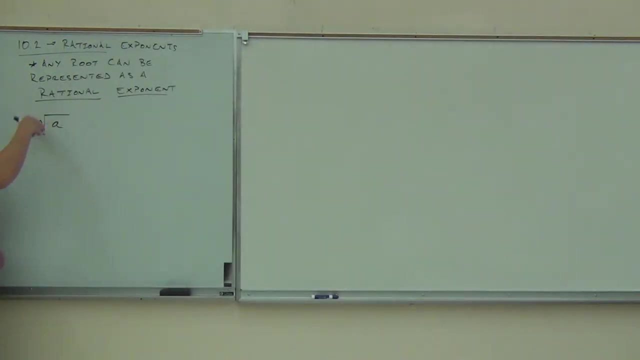 So our radicand in this case is just a. It could be anything. It could be x squared plus three. It could be whatever I want it to be. Here's the deal. This is kind of neat. Every single time you've seen something like this this actually represents. 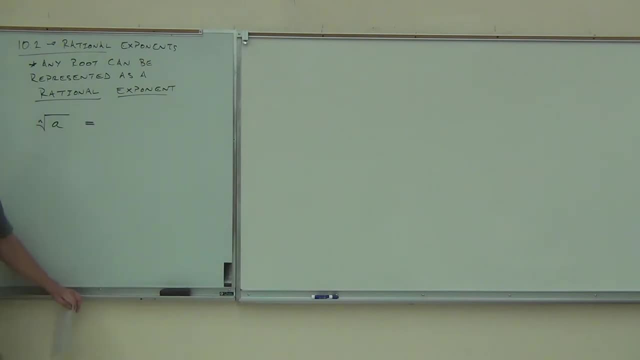 A fractional exponent, and here's how you write it. You have in this case. our base is a. It's whatever our radicand is. An nth root of a is the same thing as a to the one over n power. That's how you change from a root into a fractional exponent. 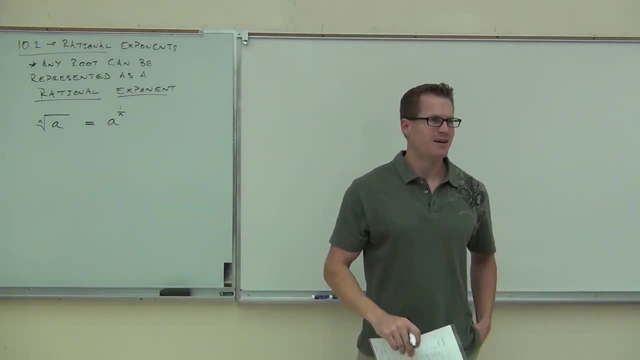 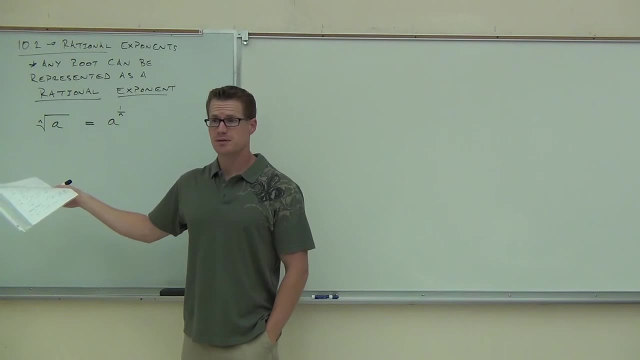 Weird huh. Why are we doing that? Why are we making these look like those? Well, I'll tell you what. Do you know anything about exponents? If you multiply common bases, you add exponents. right. If you have an exponent to an exponent, you multiply. 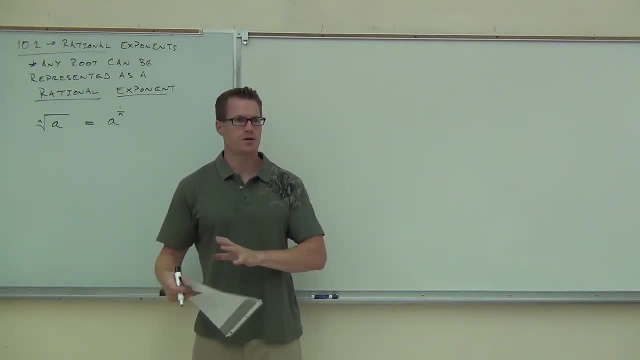 If you divide, you subtract. We can do all that stuff with our roots. now, We couldn't do that here, It wouldn't make any sense to do that, But as soon as we translate to a fractional or rational exponent, we can do all those things that you already learned. 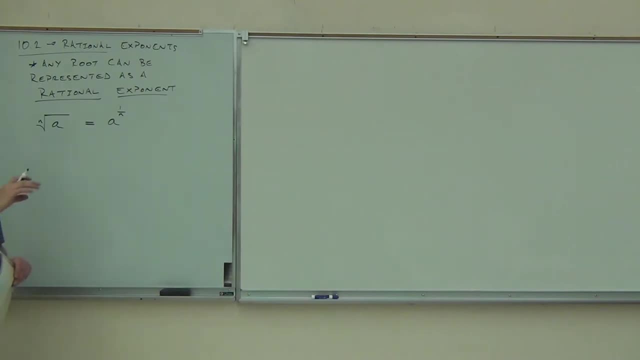 That's why we're translating these. Let's see if we can manage to change some of these from this form back into our roots. Are you guys ready to try some of this? Okay, let's do this. So first one, let's say that we had 25 to the one half power. 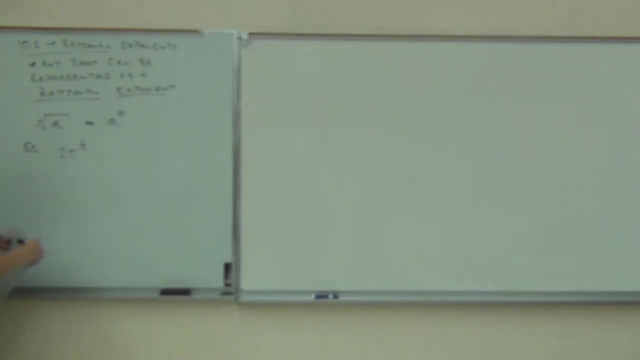 25 to the one half power. You can notice a couple things about this. Firstly, where does our n go in our fractional exponent? Where does it go? Numerator or denominator, Denominator, And where does that 1 come from? 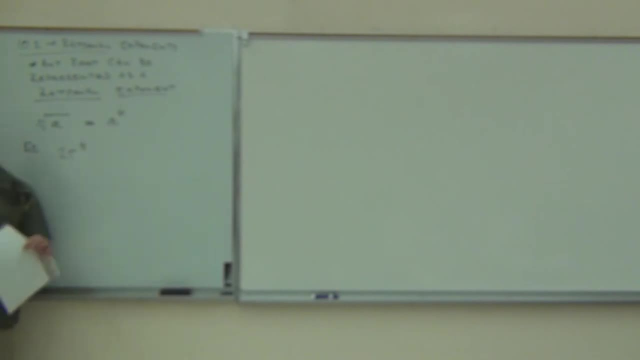 I'll show you this right now. I'm not supposed to until later, but I'm going to give you a sneak peek. okay, Where this 1 comes from. What's the power of a right here? That's where the 1 comes from. 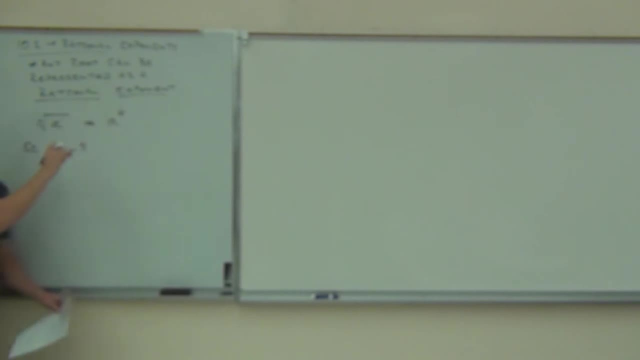 Okay, so this is a little preview of where that number comes from Right now. this is just a to the first power. That's why we have a little 1 right there. You guys okay with that? So question: can I represent 25 to the one half as a type of root? 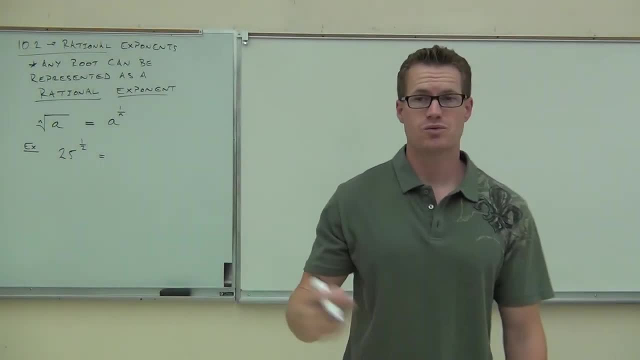 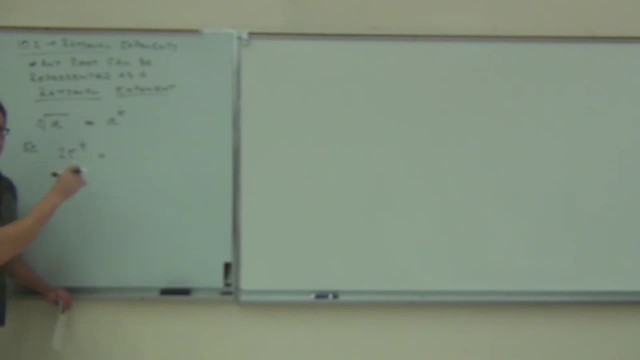 Firstly, you guys tell me what type of root is it? Is it a square root, a cube root, a fourth root? What is it? What tells you that? Yeah, that denominator right there tells you the type of root that you have. 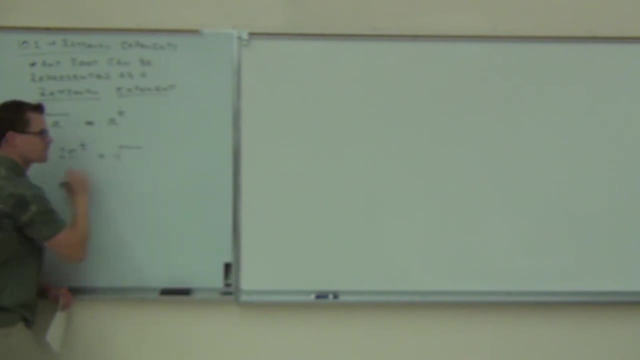 So if you have a 2 on the denominator, that means you're dealing with a square root. What's going to go on the inside of our square root 25.. 25 to what power? First, Yeah, the first power, because that number right, there is a 1.. 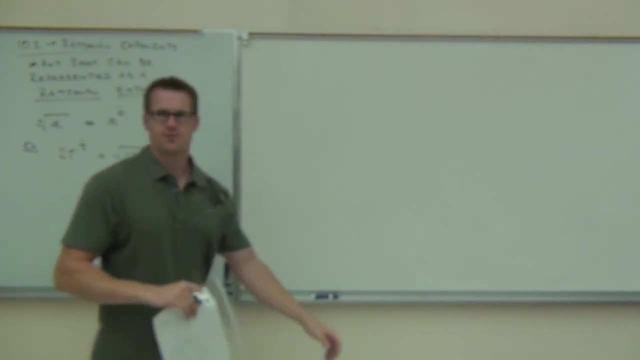 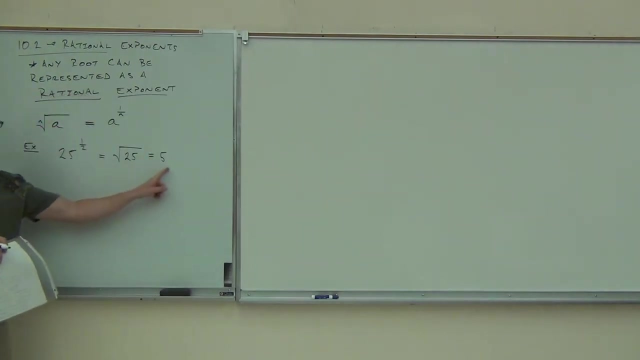 How many of you feel alright with this? What is 25 to the one half power, Or in other words, what's the square root of 25? 5. Which means that you don't have to change it to this to find that number. 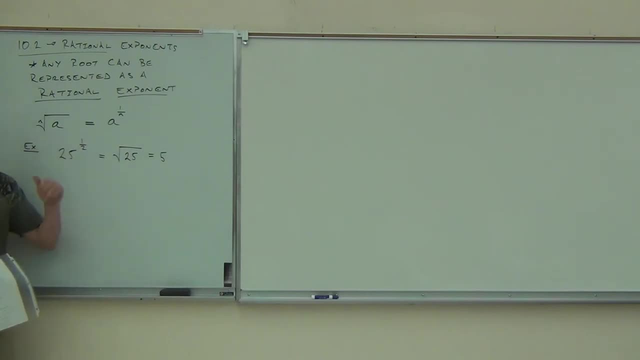 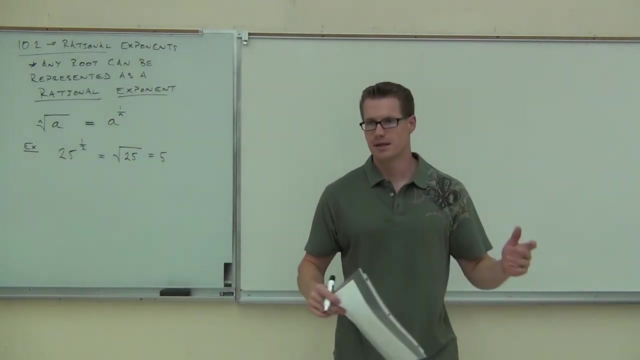 In fact, if you have a calculator you want to plug in 25 to the one half power, it will give you 5. Because it means the same thing. 25 to the one half and the square root of 25 are identical. 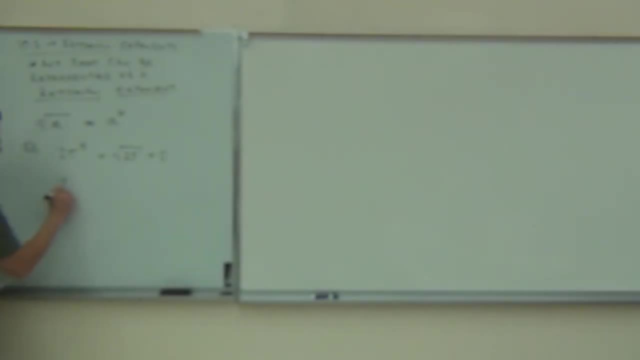 Let's try a few more. Let's try: 27 to the one third. Can you tell me, ladies and gentlemen, what type of root does this suggest? Q, Good, What tells you the Q, The denominator? Okay, so we are going to have a radical. 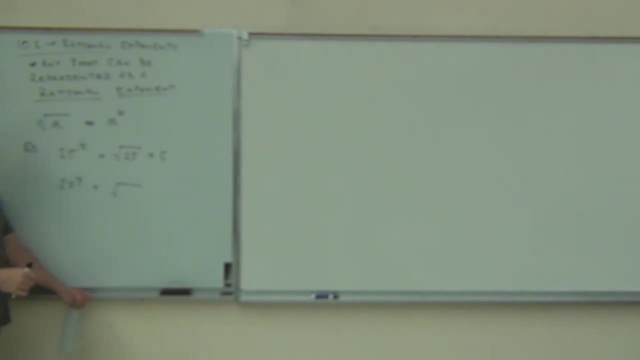 We know that any rational exponent is the same thing as a radical. We just have to make sure that our root is the same. Here is square root. Here we can't forget the 3. That's a cube root. On the inside we will have 27.. 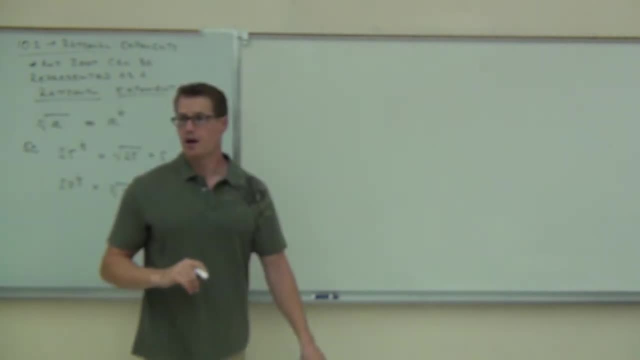 And can you tell me what is the cube root of 27?? What do you think? 3. Yeah, because 3 times 3 times 3 equals 27.. We've dealt with these roots before. We're just now translating from here to here. 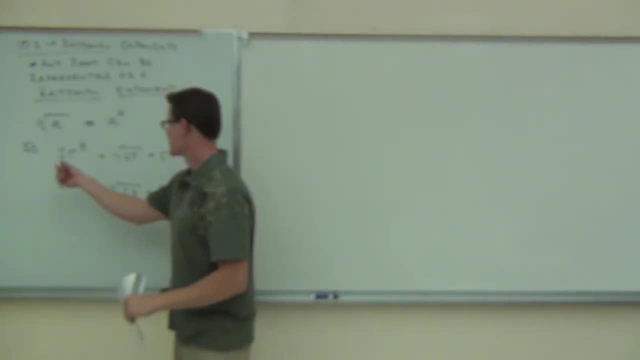 By the way, you're going to get pretty good at this- to where you're going to be able to look at these things and know immediately: oh, that's 5.. That's the square root of 25.. Oh, that's 3.. 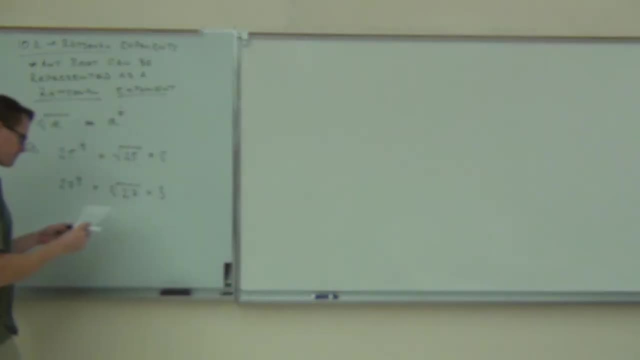 That's the cube root of 3. So you'll get pretty good at that. Can you do it with just a variable, without some numbers? Let's see if we can translate that. Ladies and gentlemen, what type of root am I dealing with? 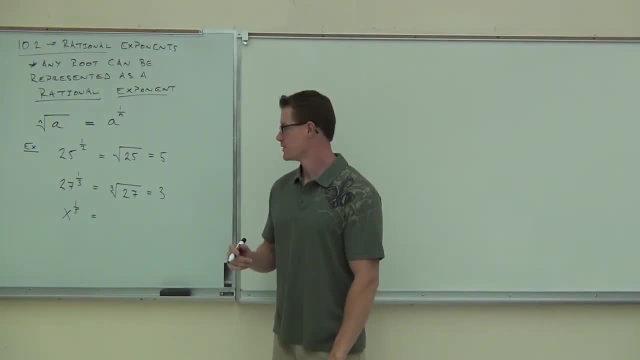 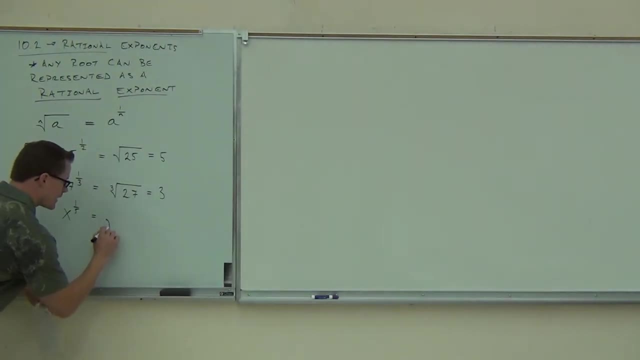 Square root. What type Fifth root? Yeah, Flipped around in your head, didn't it? Yeah, we've got a fifth root here. That's all right. So we'll still have a radical. The denominator simply tells you what type of root you have. 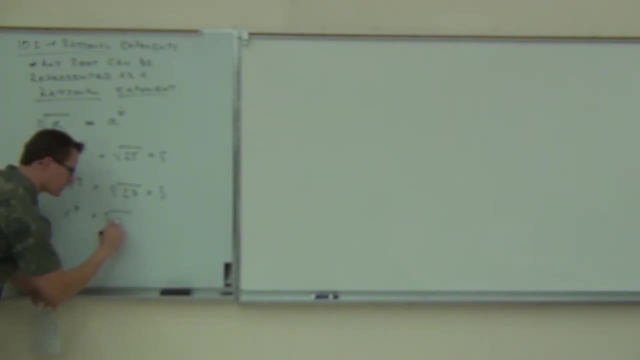 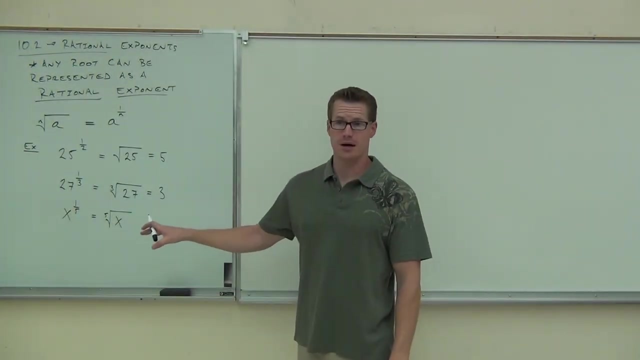 What's going to go on the inside of our root X? X to what power First? So you're going to leave it just like that. That's the fifth root of X. There's no way we can simplify that right now. 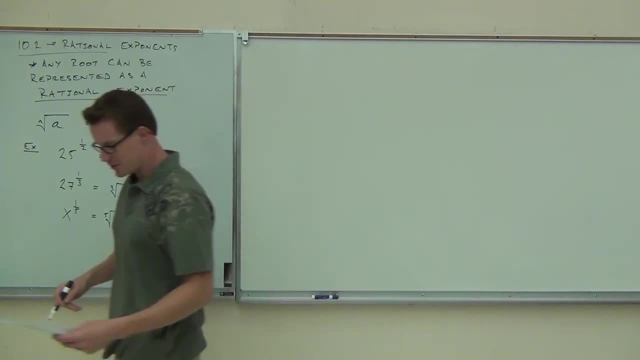 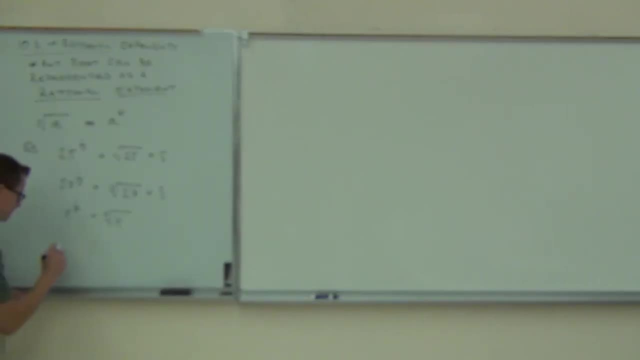 There's no number, So we can't say like here was a 5,, here was a 3.. We can't do that. Let's try a couple more. Don't answer this question out loud, but I want you to think of it, okay. 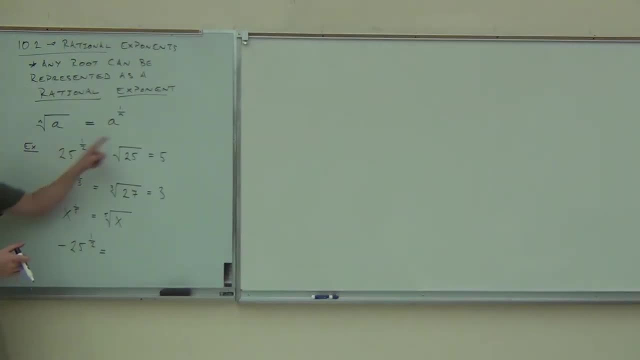 Now, of course, we're getting pretty good at this. We know that's going to be 5, and that's going to be 3, and this is the fifth root of X I want you to think of. don't answer, because I'm going to tell you the answer in a second. 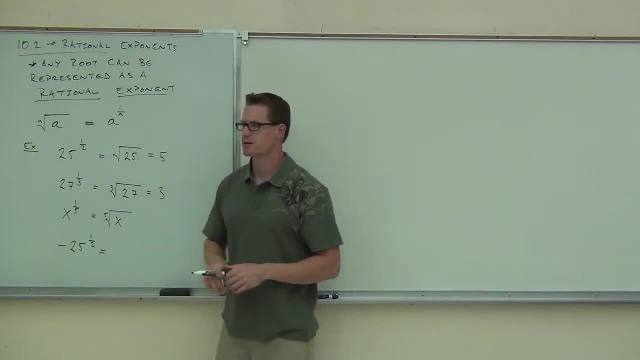 I want you to think of if this is possible or not. Don't say it out loud, Just think. I see a lot of, I see a lot of Now here's the deal. A lot of people are thinking no, right now, because you have a negative. and what type of root is that? 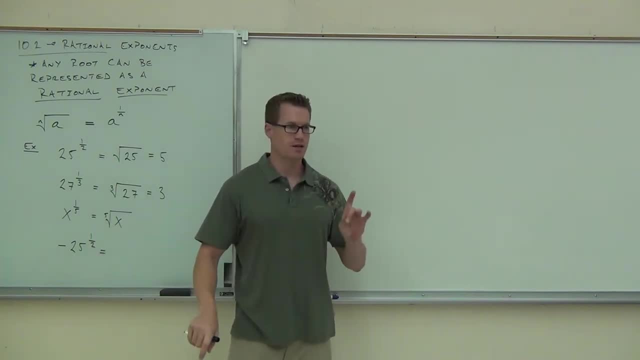 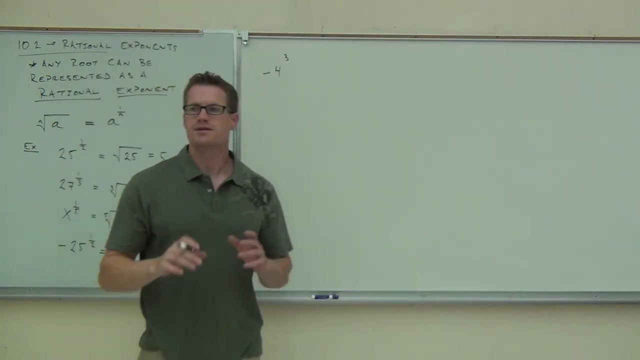 Square root And what you know is that you can't have a negative inside of the square root. Nod your head with me if you understand that for sure, But here's what you need to understand When you're dealing with exponents. if you have something like this: negative 4 to the third power- what this means. 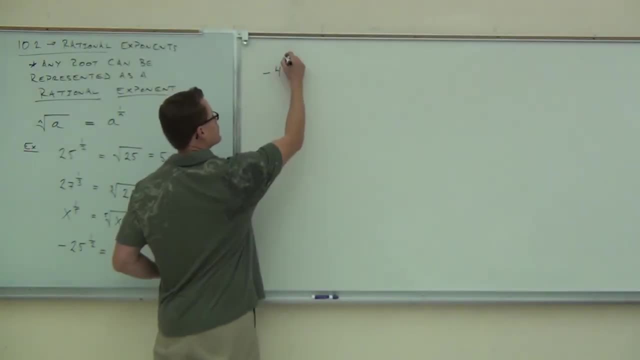 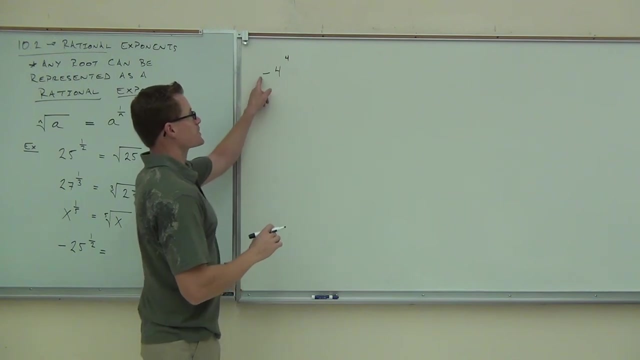 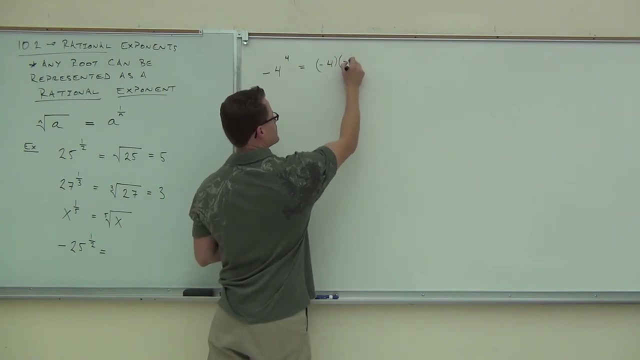 Actually, you know what? Let me make it to the fourth power: Negative 4 to the fourth power. there. What negative 4 to the fourth power means is the opposite of 4 to the fourth. What I mean by that, This does not equal negative 4 times negative, 4 times negative, 4 times negative 4.. 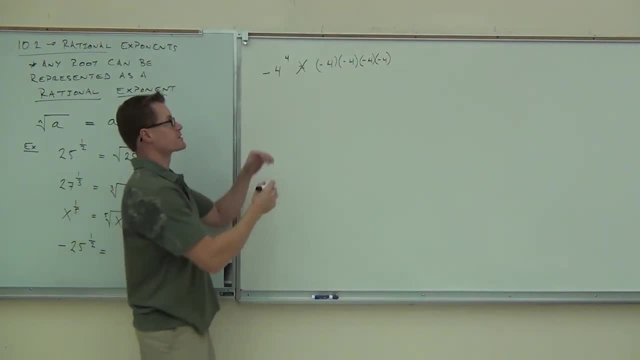 That's not the same thing. What this actually equals is Here. I'm trying to make this so you really understand it. Think of your order of operations. What comes first, multiplication or exponents Multiplication? Hopefully exponents come before multiplication, right. 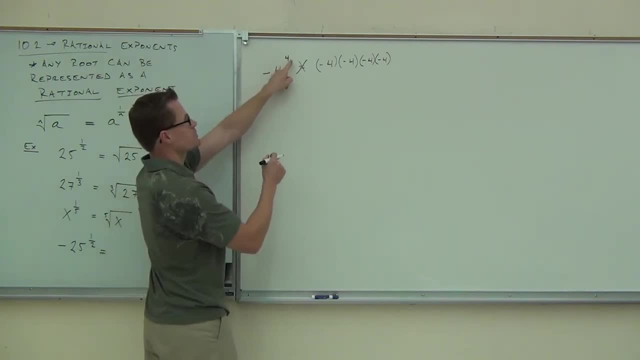 M dots. So if we have order of operations it says you're supposed to do your exponents before you do any multiplication. So what this actually can be written as. pay attention up here you could write this as negative 1 times 4 to the fourth. 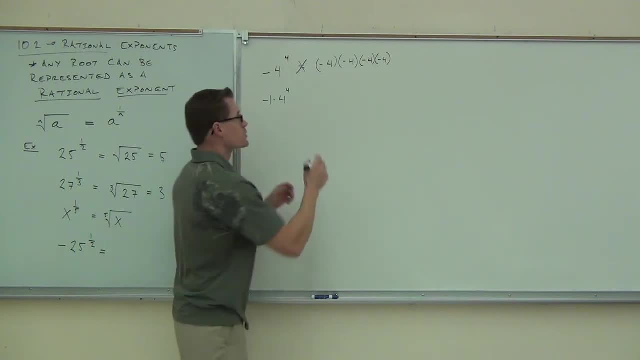 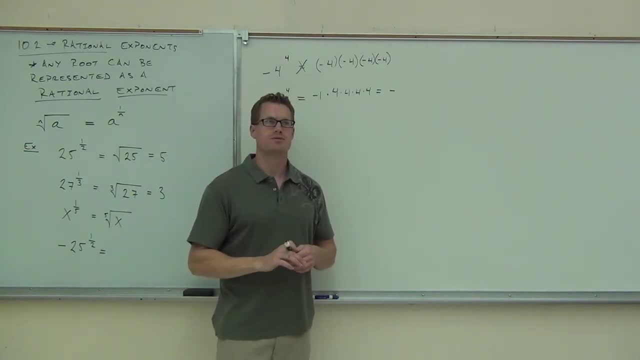 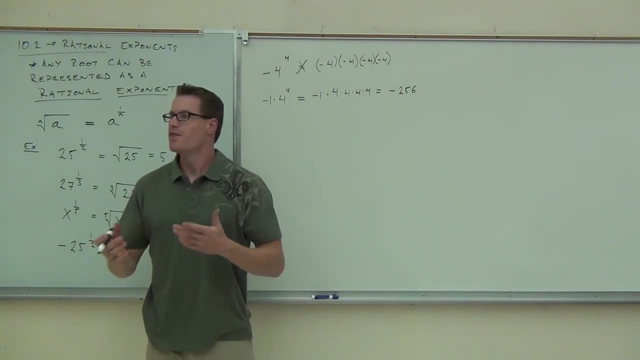 Negative 4 to the fourth. 64 times 4: 256? Negative 256.. So even though you have a negative 4 to the fourth power, you're still getting a negative. Are you guys okay with this? 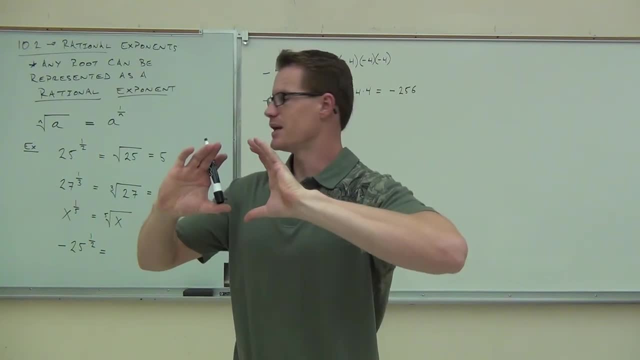 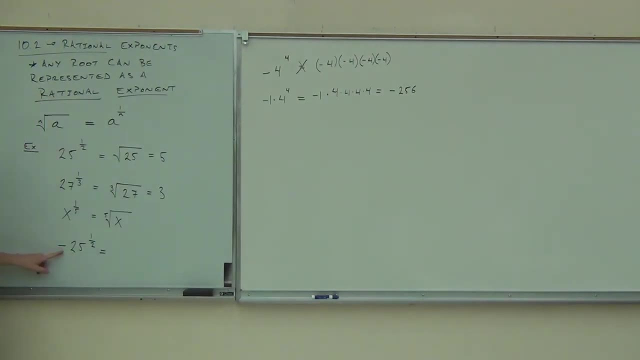 Here's what I'm trying to say. Unless your negative is in parentheses, it is not being applied towards that exponent. Are you with me? So in this case, is this negative 25 going to be inside of the square root or is it going to be outside of the square root? 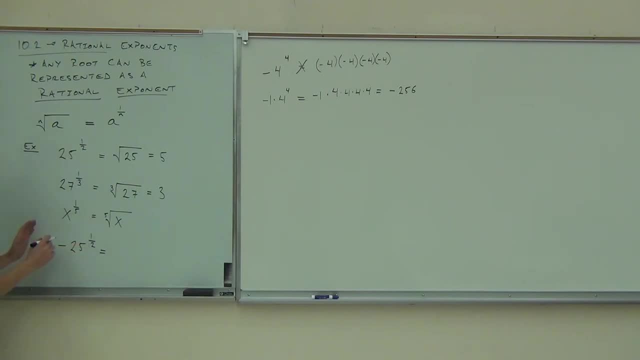 Outside. It's going to be outside. yeah, How I would show it inside is if I had this Watch on the board. If I had that, then it would be inside the radical. Are you with me If I don't have that? 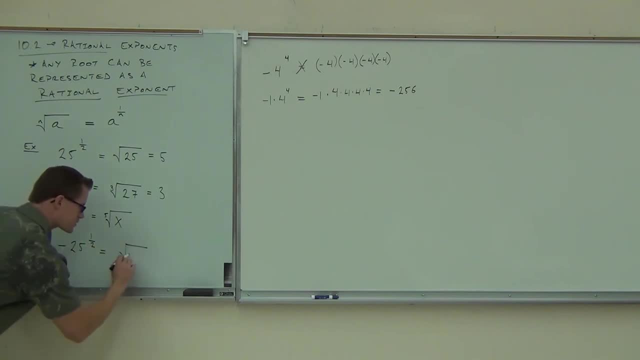 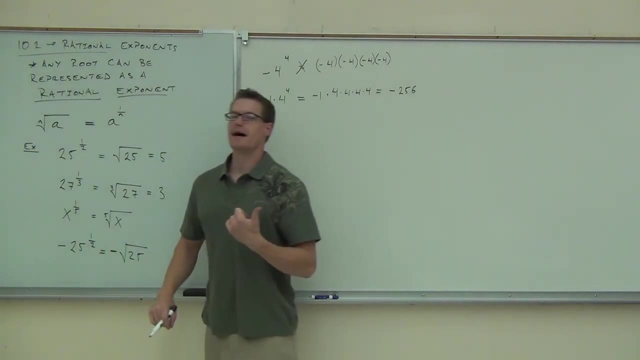 Very important that you get this, by the way. If I don't have that, then it says a square root of 25.. This is the opposite of the square root of 25.. That's what that is. Is that possible? That is definitely possible. 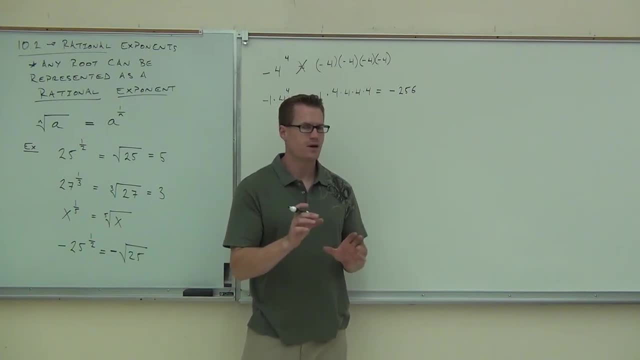 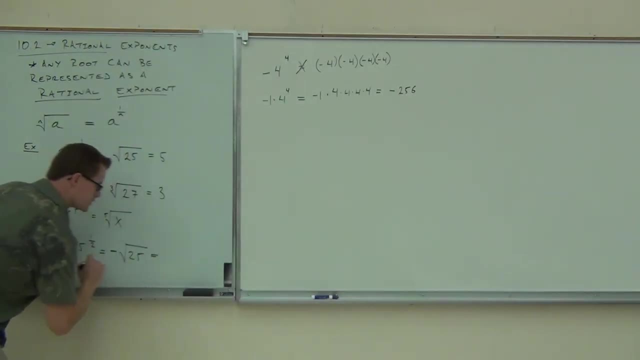 Do you see the difference here? Okay, so that negative, if it's not in parentheses, it will not be inside of the radical, If it is in parentheses, then it will be. This one is actually equal to how much Negative 25.. 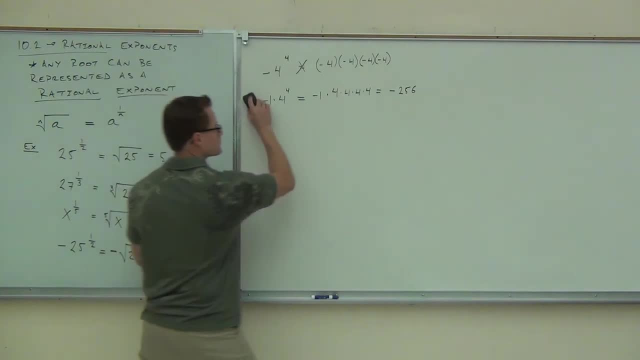 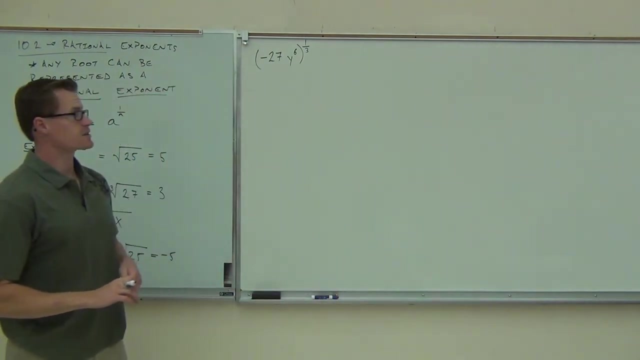 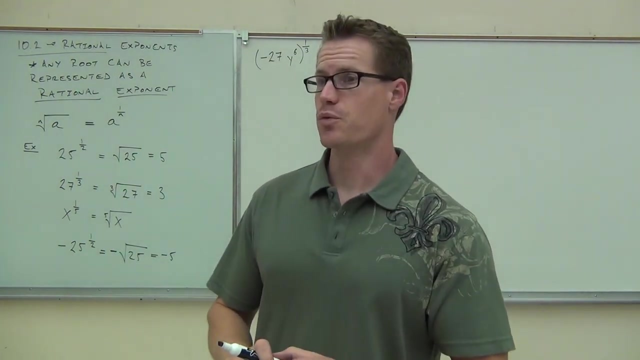 Yeah, perfect. Yeah, let's try a few more with that in mind. Negative 27,: y to the sixth, all to the one-third power. Firstly, I want you to identify if we have a root here. Do we have a root? 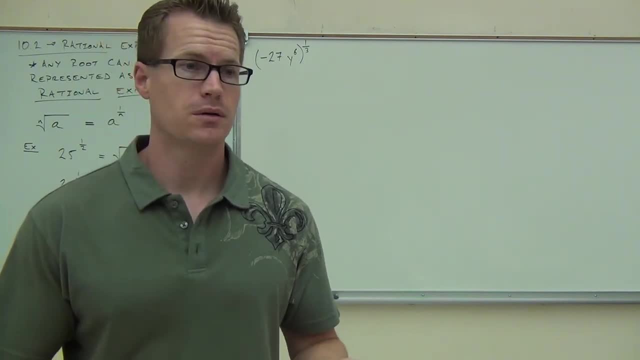 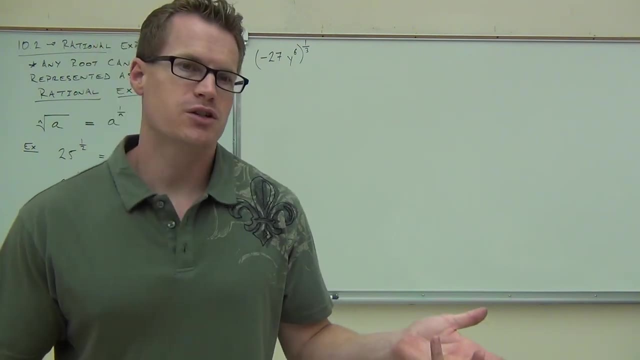 A radical. What tells you I'm going to have a radical here? What type of exponent do we have? Fraction exponent- Okay, good, So anytime you have a fraction exponent, it means a radical, for sure. What type of a radical do we have? 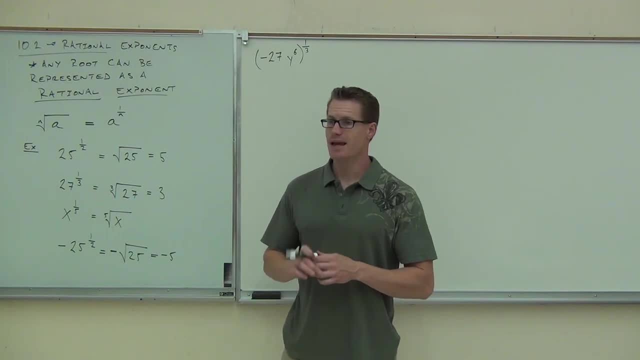 What type of root? Cube root, Cube root, All right, And is the negative going to be inside the cube root or not? Inside, Inside, Inside or not? Yeah, Why? Because of the parentheses, I want you to notice the difference. 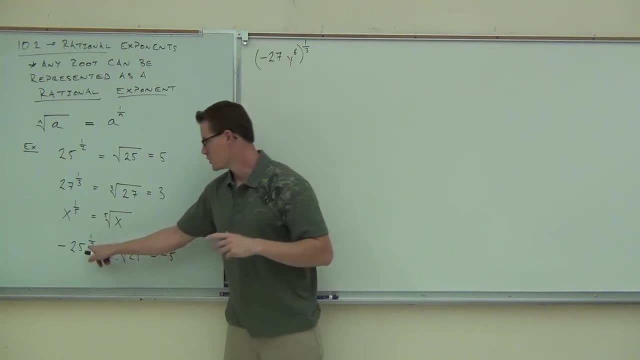 Here there's no parentheses. It's outside. Use your word operations that idea Exponents come before multiplication. This is being multiplied by negative one Here because it's in the parentheses. this says: oh okay, I have the cube root. 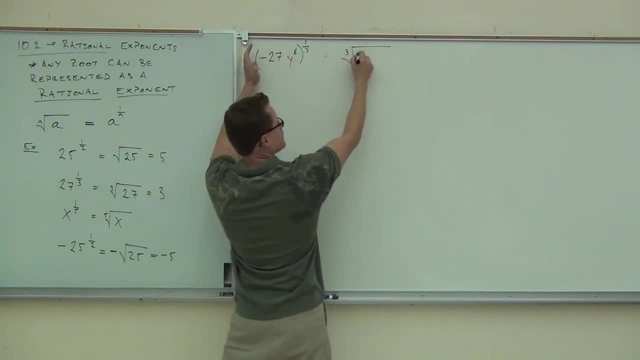 Sure, But since this is all connected with those parentheses, that's negative. That's going to be inside of my radical. Raise your hand if you feel okay with that one. Okay, I'll show you how to simplify those in a little bit. 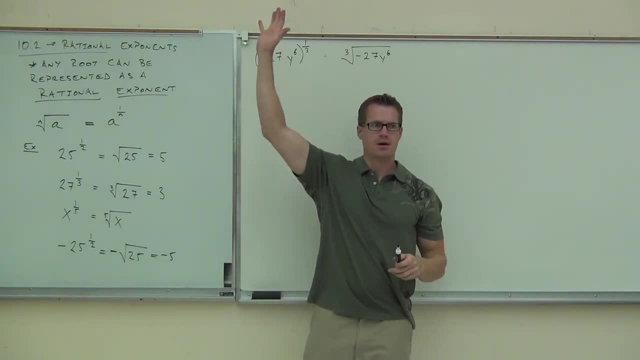 We're not going to quite go through that. Well, I guess we could. actually We could do that. now Let's simplify that. Do you remember how to simplify those from the very first section we did in this chapter? I hope so. 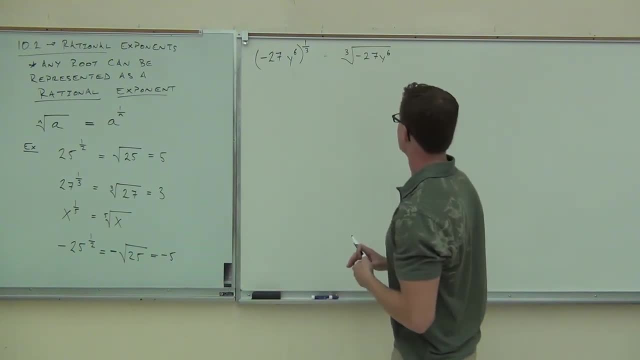 Do we know how to do the cube root of negative 27?? Sure, How about the cube root of y to the sixth? Do you remember how to do that? There's two methods. You would write this as negative. You would write this as negative. 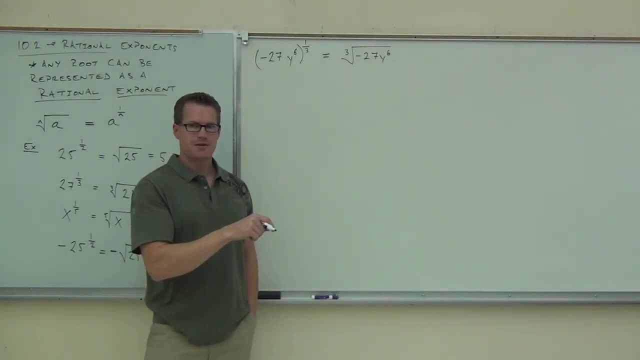 You would write this as positive. You would write this as negative. You would write this as negative. You would write this as positive. You would write this as negative. You would write this as positive. You would write this: asihad. I hope so. 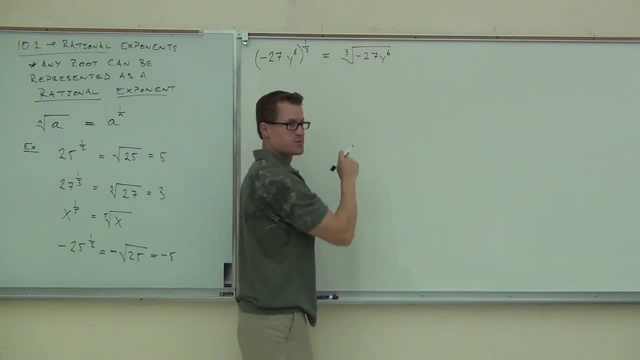 Do we know how to do the cube root of negative 27?? Sure, How about the cube root of y to the sixth? Do you remember how to do that? There's two methods. You would write this as something to the third power and cross those out, or you would write: